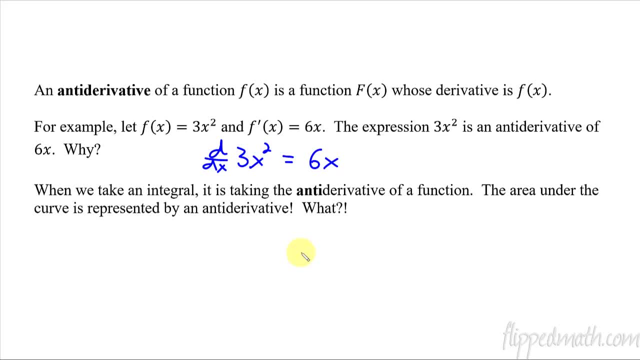 Now here's what's really weird about this: An anti-derivative within an integral, it represents the area under the curve. When we are taking an integral from a to b of some function, that is actually taking the anti-derivative And the anti-derivative would. 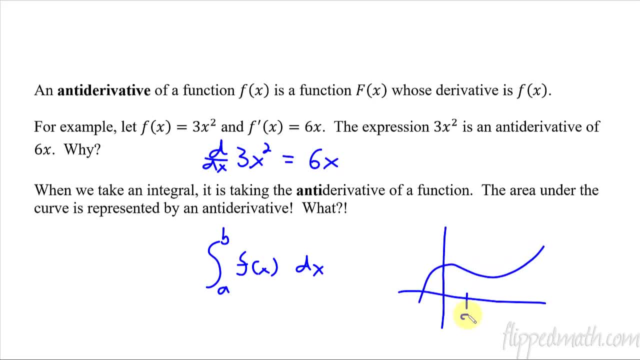 represent the area under the curve from a to b. That is the. the anti-derivative helps us get that. That's a really weird connection Like: why does that work? It's not even something that was intuitively seen by Isaac Newton and Gottfried Leibniz way back when they were first studying. 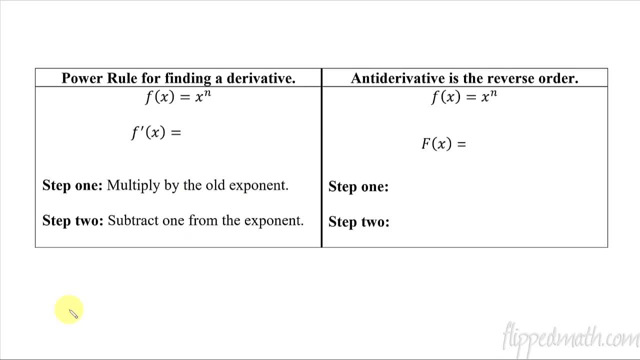 what this calculus stuff was all about. They didn't even see that at first. So let's talk first about power rules. So let's talk first about power rules. So let's talk first about power rules And then how you take the anti-derivative. So power rule. if you remember, we would do this. 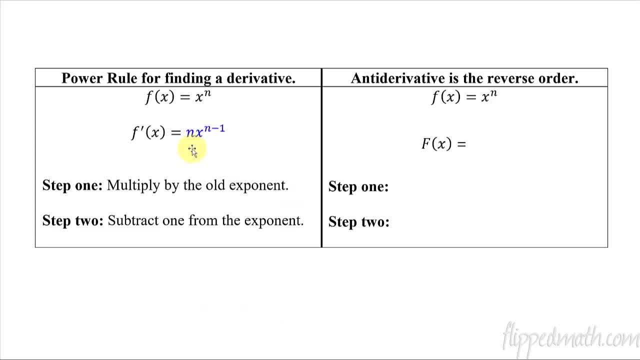 already. You know how to do this: Multiply by the old exponent, just bring it down to the front, and then you subtract one from the exponent, So there's our new exponent. All right, Now, if I'm doing anti-derivative, I'm going to swap these steps and do the inverse of them. 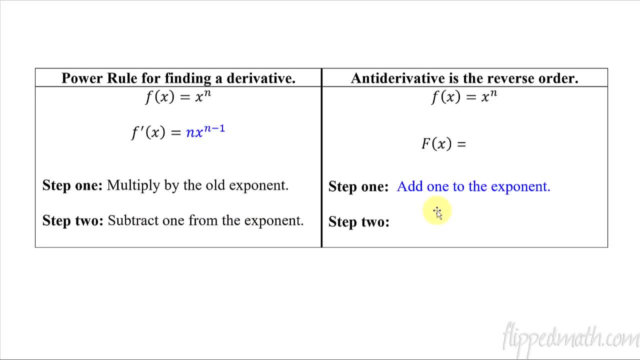 So, instead of subtracting one from the exponent, I add one to the exponent. And then step two is the power rules, step one where we now, instead of multiplying, we divide by the new exponent. Okay, So those are our steps for taking the anti-derivative. So you think, here you add one to 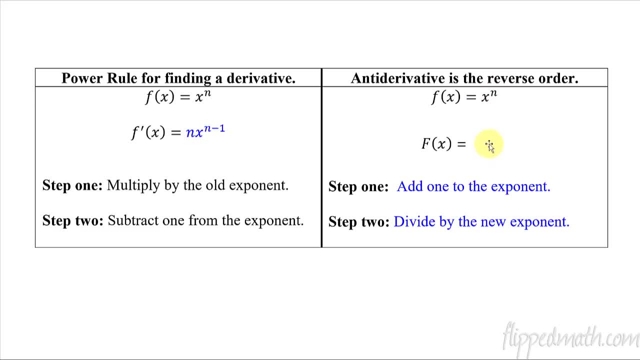 the exponent adding one, and then you divide by whatever that new exponent is. So it will look like this: x raised to the n plus one, all divided by whatever that n plus one is. All right, So get that written down and let's jump into examples. So I'm going to find the anti-derivative of this. 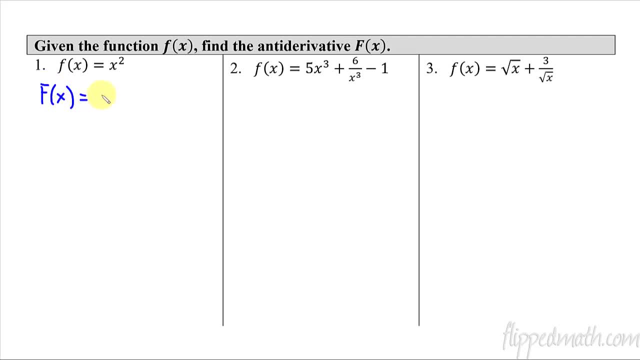 That'll be my capital F of x And that's going to equal. I take x squared, I add one to it, So now it's three, And then I divide by that new number three And then I have to do a plus capital C. This capital C stands for a constant. 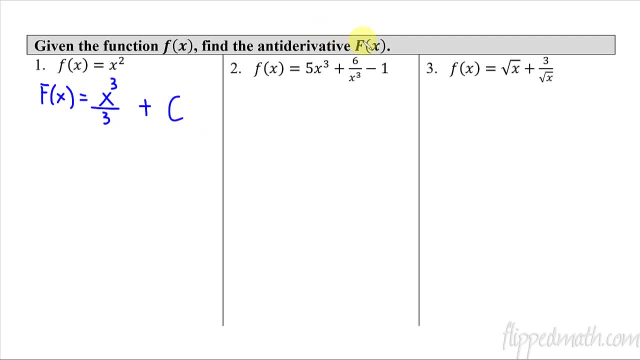 any constant I want. Now I have to include that when I'm finding the function. that's an anti-derivative, because- and we'll talk more about this next lesson- Okay, I'm just briefly talking about this C right now, but that's because any number this is, if you take its. 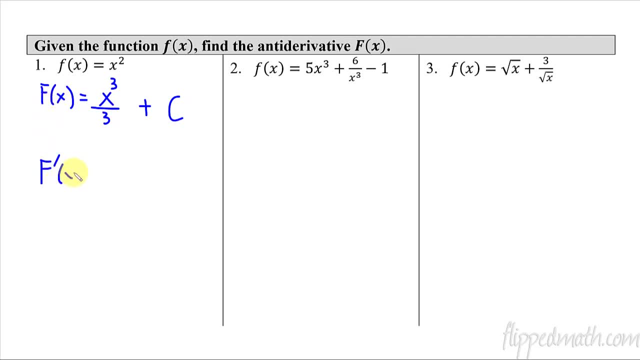 derivative. so now let's go down. and what's F prime of x? its derivative would be three. comes down, cancels. with that three x squared plus, the derivative of any constant is zero. So that would then lead us back to where we started. So that's why we put the plus C. 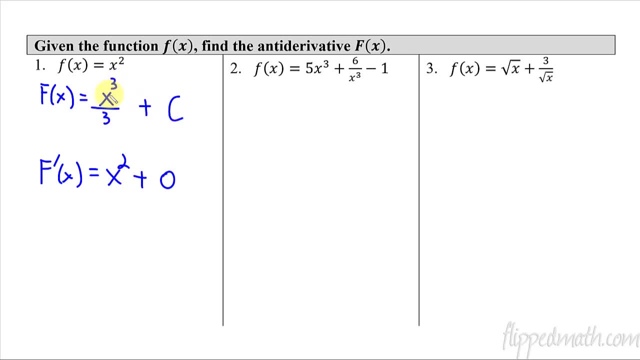 It's just to represent all families of functions that could be this. So plus any. so there's actually an infinite number of answers, depending on what this C value is. All right, So let's do this one. So before I take the anti-derivative, I'm first going to rewrite this F of x as five. 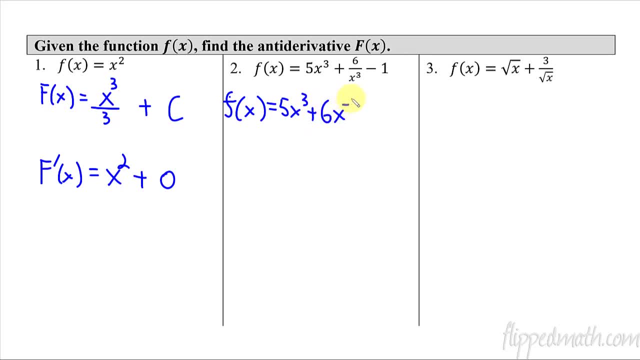 x, cubed plus six, x to the negative, three minus one. This is like when we did the power rule with derivatives. it helped to rewrite it, So let's do that, So let's do that, So, let's do that, So let's. 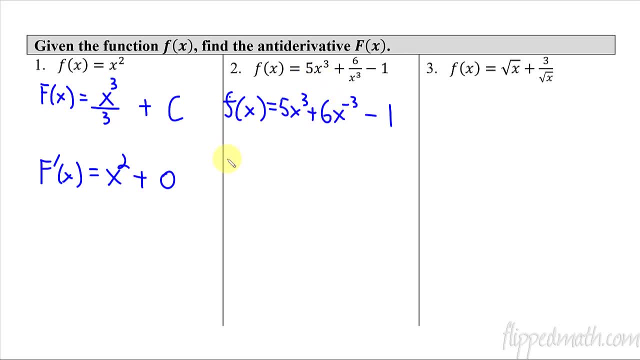 rewrite it first. It's the same with anti-derivatives. If you want to rewrite it first to be able to tell what our exponents are, it might help just a little bit. So now we add, so it's going to be five x to the. add one fourth and then divide by that number four plus six x to. 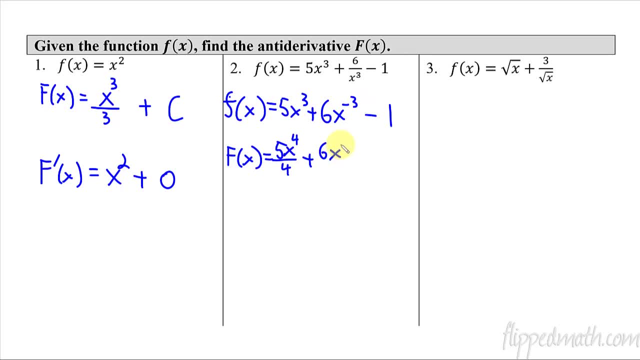 the add one. Remember you're adding to a negative number, So that's negative two. Big mistake here is when you make that a negative four. kids do that all the time. That's wrong. And then you divide by what that new exponent is, So that's negative two. And then 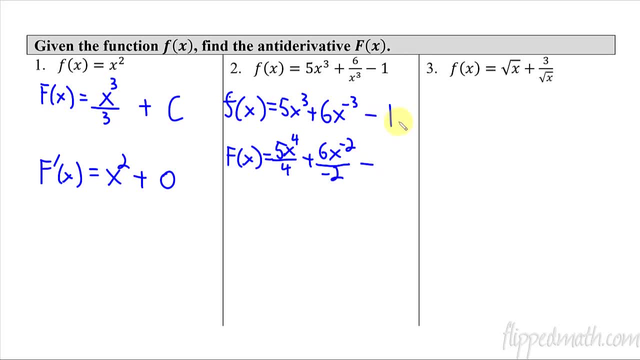 minus. how do you take the anti-derivative of a constant? Well, you just have to think. this is like the derivative answer. What's the anti-derivative of that? It's x, because the derivative of negative x would get you back to negative one. So when it's a constant, you just 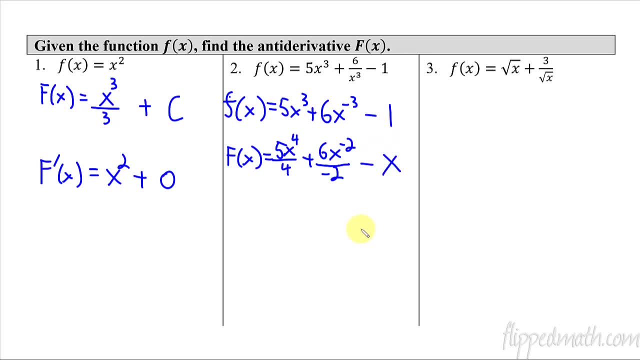 throw on that, That is the coefficient of x. Okay, now can we clean this up a little bit? Yeah, I think we can. So oh, plus c, forgot the plus c. So our F of x equals five force x to the fourth. 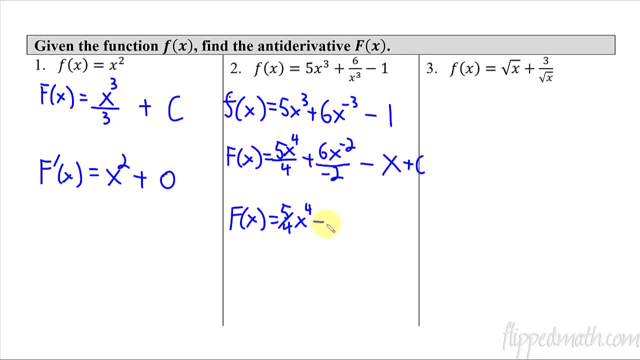 and then here we have a minus because that negative two, so minus. on top we'll have a three, six divided by two, and on bottom we'll have our x squared minus x, plus some constant c. And then the last one of this set of examples. let's rewrite this first, before we take the anti-derivative. 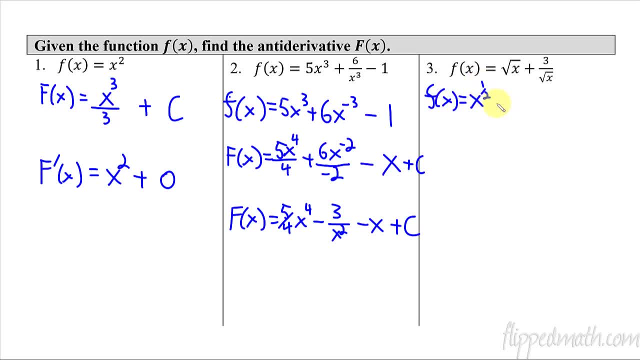 So F of x equals x raised to the one half plus three x raised to the negative one half. Okay, add one to that exponent. It's x raised to the adding one makes this three halves. add one full two over two And then we have to divide by three halves plus three x to the add one to negative. 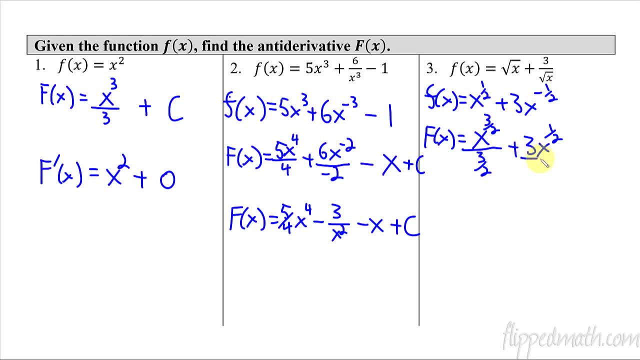 one half and you get a full one half positive, And then divide by that same exponent, one half, and then I'll add my constant at the end here, plus c. So this is weird. I hate it when I got fractions inside of fractions. so don't treat it like that. Let's rewrite this: 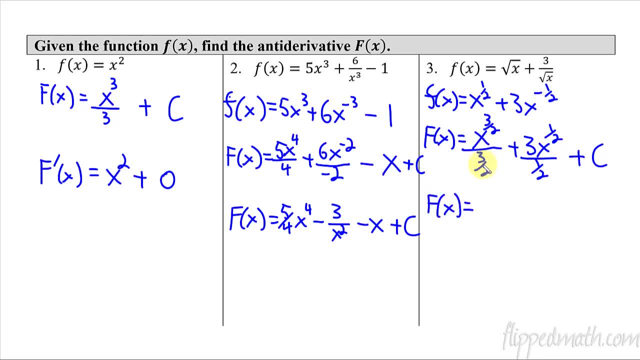 to hopefully make a lot more sense, You don't divide by fractions, you multiply their reciprocals. I'm going to multiply by two, thirds x raised to the three halves plus, and then again here, instead of dividing by one half, I'll multiply by two. So it's three times two is six. 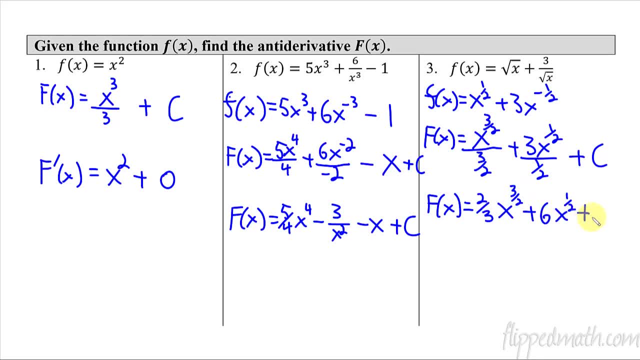 x to the one half. or you could have written square root of x plus my constant c, And there's my answers. So this rule is vital to understand before we go on to do the rest of these integrals. You've got to know how to take this anti-derivative step with these, adding one to the exponent. 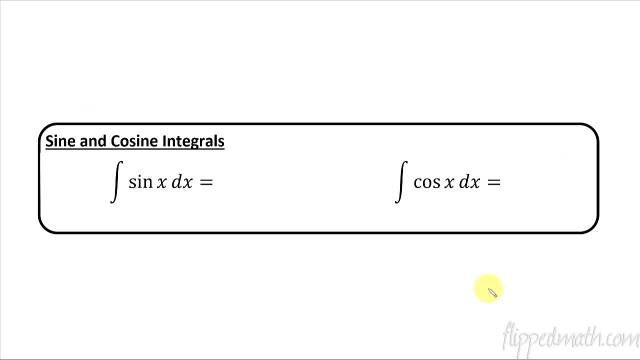 and then dividing by two. So you've got to know how to take this anti-derivative step and then dividing by that same number. Now to something where hopefully you don't start getting confused: The anti-derivatives of sine and cosine or the integrals of sine and cosine. 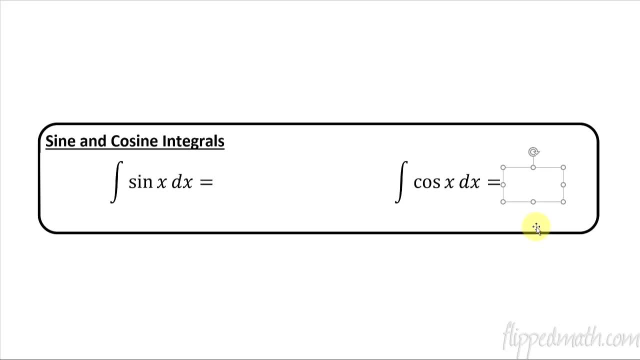 So let's start with this one. it's a little easier. This one is what's behind my little white box here: Cosine of x. What would the derivative be? What do I take the derivative of to get an answer of cosine. Well, that's just sine. Oh, I've got to add my plus c, Whoops, Plus. 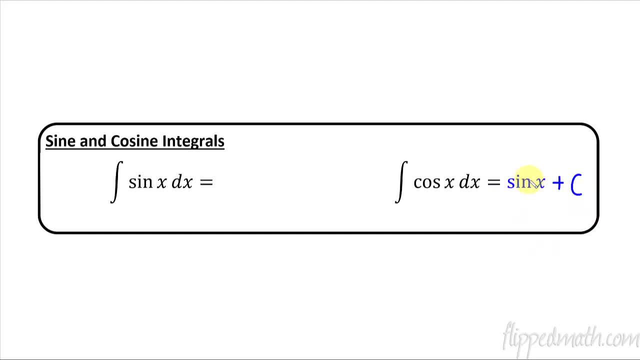 some constant. I've got to put a plus c there, So sine of x plus c, that would be the anti-derivative of cosine x, Because the derivative of sine is cosine. So now that leads us to this one, which is a little. 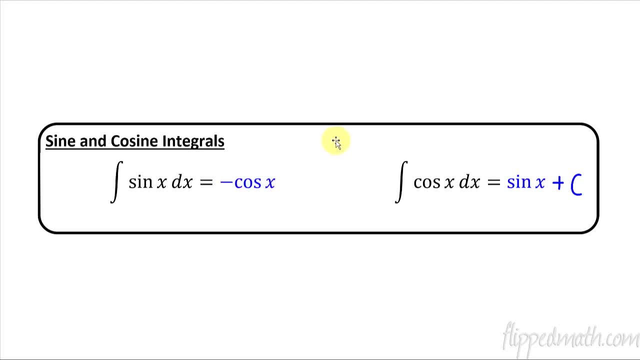 different. This one would be negative cosine of x and then add my plus c. Now why negative? Because the derivative of cosine- remember The derivative of cosine x- is equal to negative sine x. So if I was taking the integral of negative sine x, I would get cosine x. If I'm taking the 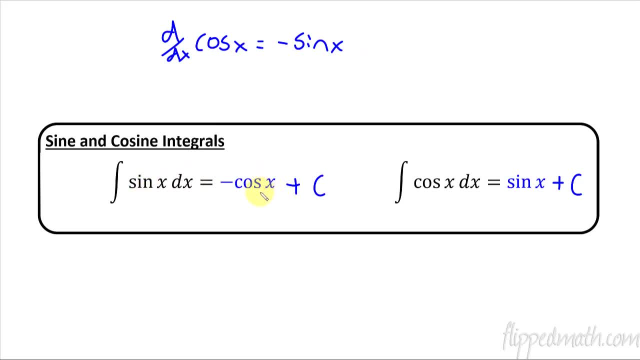 integral of positive sine x, it would have to be negative cosine x. Right, Because if I took the derivative of negative sine x, I would get cosine x. So if I took the integral of negative sine x, that would then give me positive sine x. So that's where that comes from. Again, don't get confused. 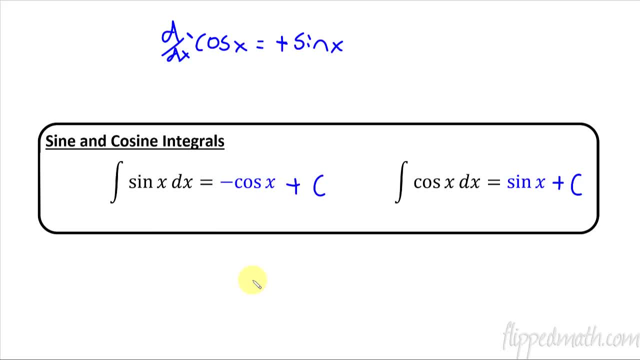 with how the memorization works. I find it easiest for most students if they just keep the memorization of the derivative and then here they work backwards to make sure that it works, And you can always, when you're done, you take the derivative real quick just to see if you did it. 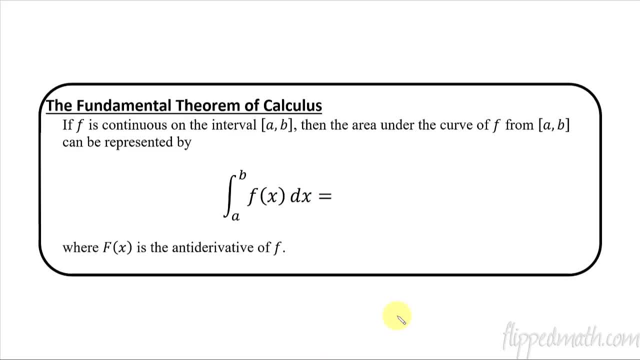 right, All right. now it leads us to the Fundamental Theorem of Calculus, part one. Remember, earlier in the year I talked about the Fundamental Theorem of Calculus a few lessons ago and we did part two. That's because most textbooks do this one first. They'll talk about this as part. 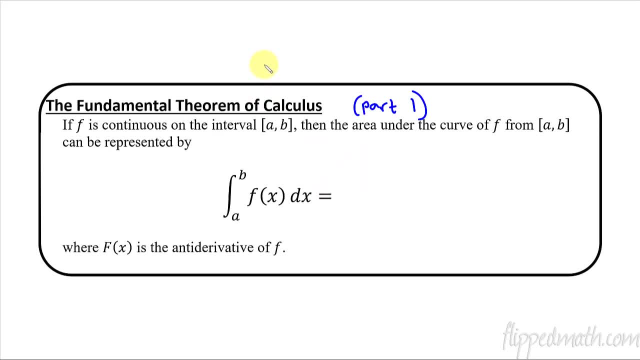 one and then later on they'll get to the other part of the Fundamental Theorem of Calculus. All right, so here we go. If f is a continuous function on this interval a to b, the area under the curve is this definite integral. We've already talked about that in several lessons. that that's. 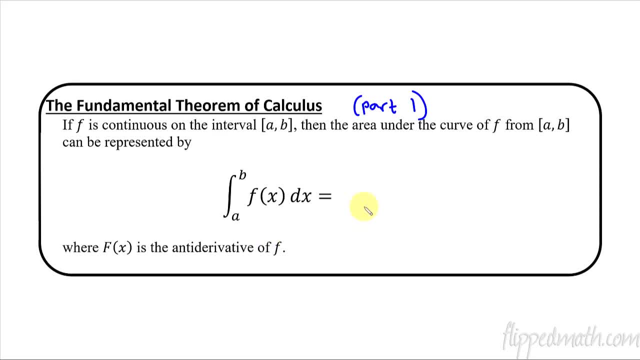 what this represents. But instead of doing summation, notation and a long crazy thing, there is a way to do this fast, And that is you take the antiderivative capital f, you plug in the upper bound b and then you subtract the antiderivative with the lower bound a plugged in, And then that. 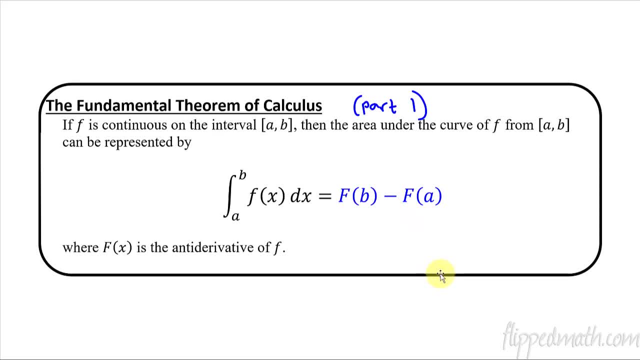 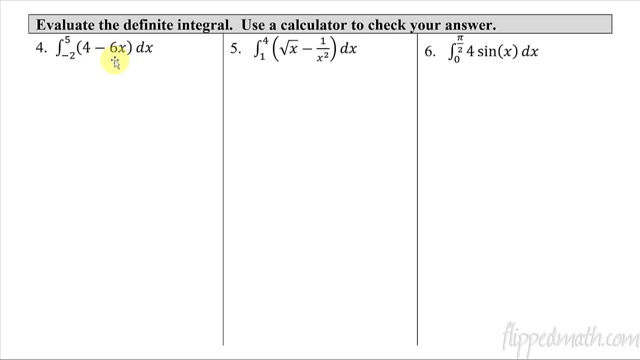 represents our area under the curve. Okay, so get that written down and let's do it. So we're talking about this function: 4 minus 6x, It's just some straight line, the slope of negative 6. And we're talking about the area under the curve from negative 2 to 5, so the area between that. 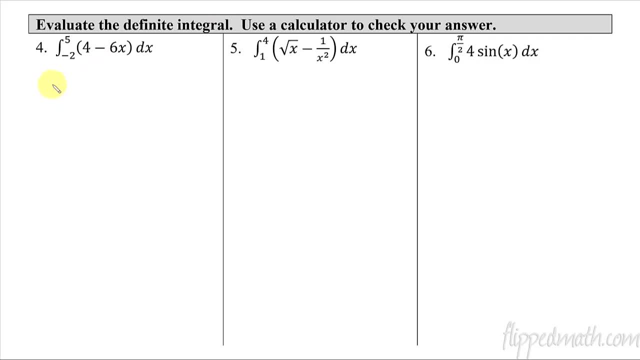 and the x-axis. So the way we do this is we're going to take the antiderivative first, So I'll take the antiderivative of 4 as 4x. Why? Because its derivative is 4.. And then, minus, we take 6x. 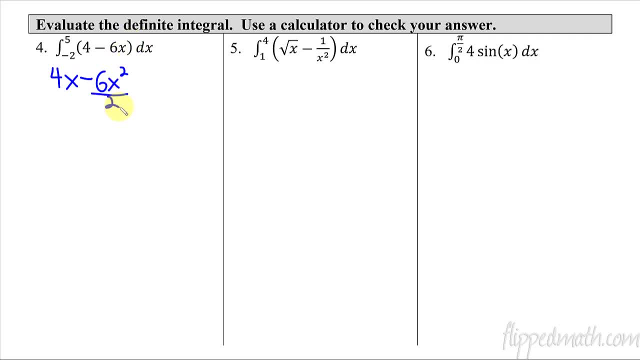 add 1 to the exponent, so now it's squared, and then divide by that same number, 2.. And then I'm going to draw a line over here And this line- there's lots of ways that you might see it- and 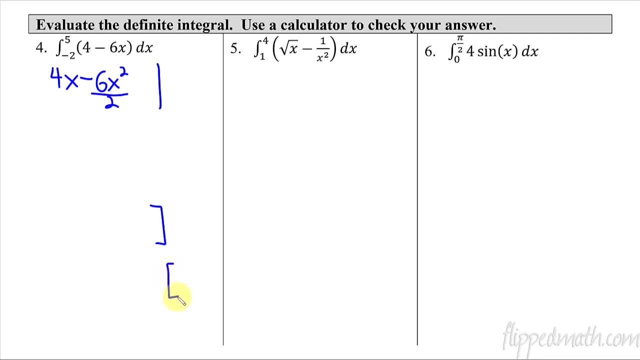 sometimes textbooks will do brackets. Sometimes they'll maybe have a little bracket. this way They'll do it all sorts of different ways. Most of the ways I've seen it is just a quick little line. So we're going to do this line from negative 2 to 5.. This little line just is a placeholder. 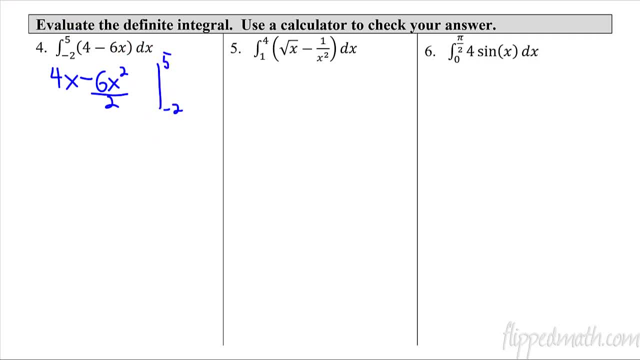 To remind me that I'm I still haven't plugged in my boundaries. I should mention real quick, I know I did not put a plus C for my constant of that antiderivative, but that's because you'll see in just a second it would cancel out Those C's. the C would be totally gone. here I'll show. 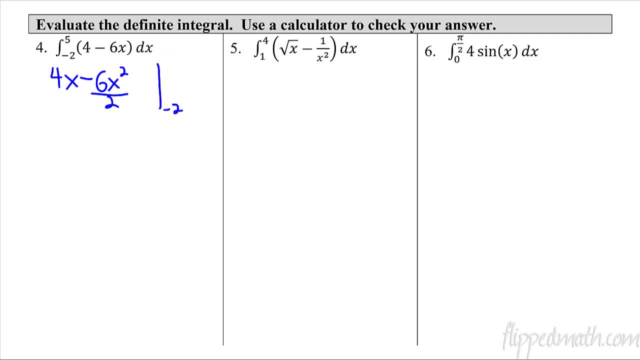 you that in just a minute. So what I'm going to do and actually is write my 5 in red so that you can kind of see the difference of what I'm doing here. So I will first plug in the 5. The 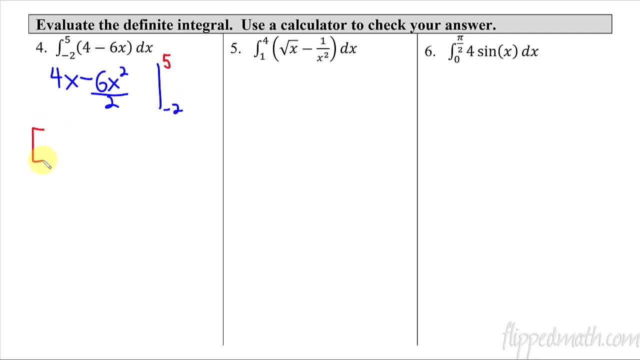 upper boundary goes first. So I will say bracket 4 times 5 minus 5.. And then I'm going to do this minus, and now this is just 3, right, 6 divided by 2 is 3.. So it's 3x squared, So it's a 5.. Okay, 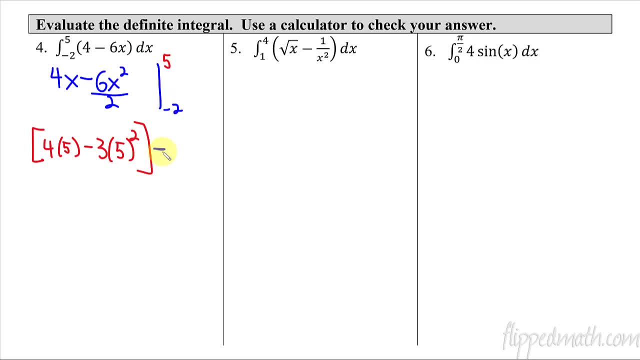 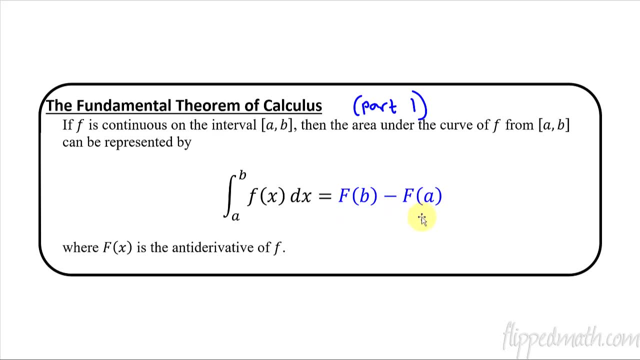 So that whole thing is just a 5 plugged in. Now I subtract. Why am I subtracting? Because that's the fundamental theorem of calculus. I do the antiderivative with a B plugged in, minus antiderivative with an A plugged in. So now plug in that A and I get. let's do my brackets here. 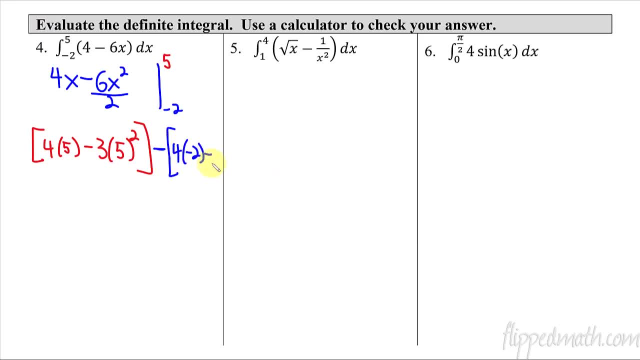 4 times negative 2 minus- I'm trying to write small because I'm running out of room- 6 divided by 2 again, was 3.. So I have 3 and then negative 2 squared. Oh man, sorry, I went over to number 5.. Okay Now. 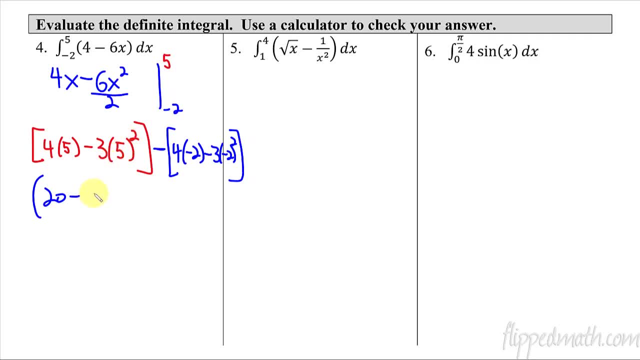 simplify this up: 20 minus 5, squared 25 times 3, 75 minus open parentheses, 4 times negative, 2, negative, 8 minus 3 times positive, 4, 12, negative, 55 minus a negative 20.. So that actually makes. 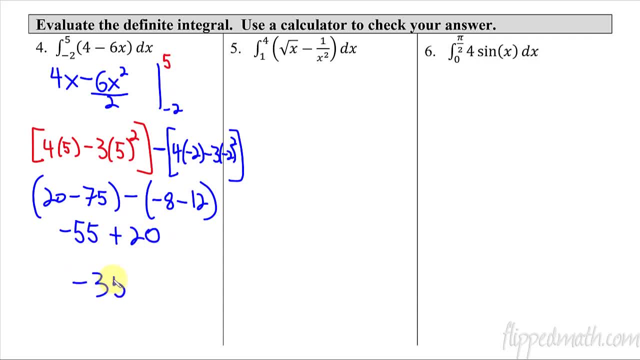 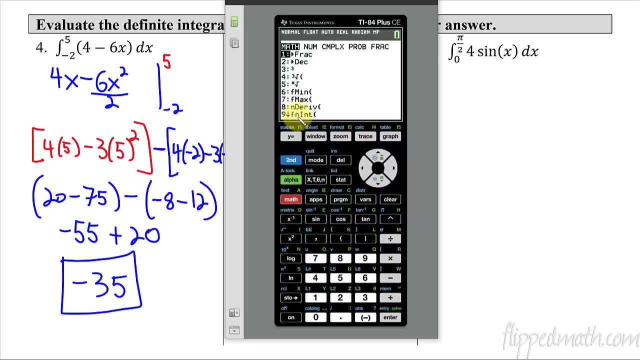 it plus 20.. And then that leads us to negative 35. Now let's check with our calculator See if this worked. So I'm going to type in the math menu and then option number 9 is the integral, 8 was the derivative, 9 is integral, Let's do 9.. And then I'm going from negative 2 to 5.. So we go. 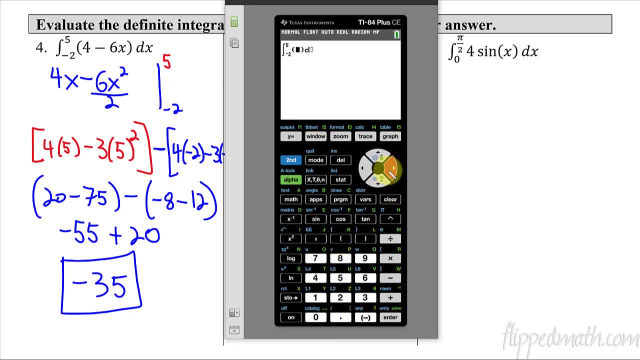 negative 2 up to my upper bound of 5.. And I have to type in 4 minus 6x, And then that's all with respect to x. Enter negative 35.. Okay, good, So we've got that one right, We did it, So let's go. 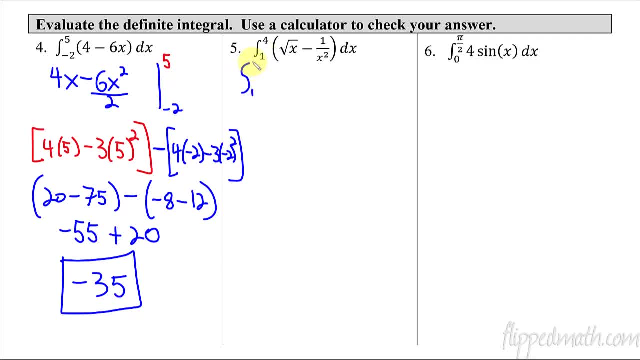 on Now, before I try to take the antiderivative, let's rewrite this, because it will help me out If I can see the exponents: x to the 1, half minus, x to the negative, 2 with respect to x. Okay, 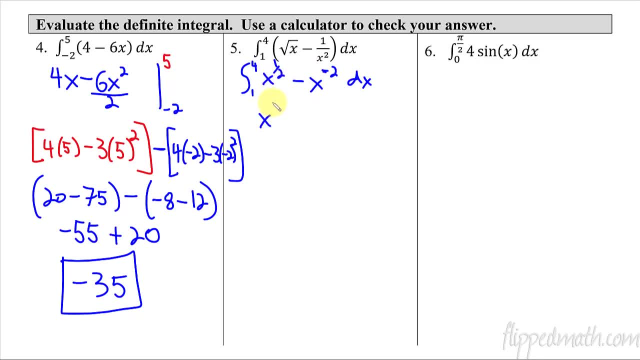 so now the antiderivative is add 1.. I get x raised to the 3 halves, all divided by 3 halves minus x to the add 1.. I get negative 1, all divided by negative 1.. And then I'm evaluating it. 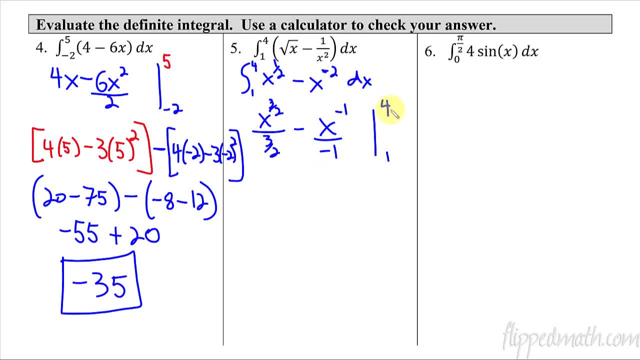 from 1 to 4.. And the upper bound gets plugged in first. Before I do this, I'm going to simplify this even more. So this is 2x. I'm going to simplify this even more. So this is 2x. I'm going to simplify. it even more. So this is 2x. I'm going to simplify it even more. So this is 2x. I'm going to simplify this even more. So this is 2x. I'm going to simplify it even more. So this is 2x. I'm going. 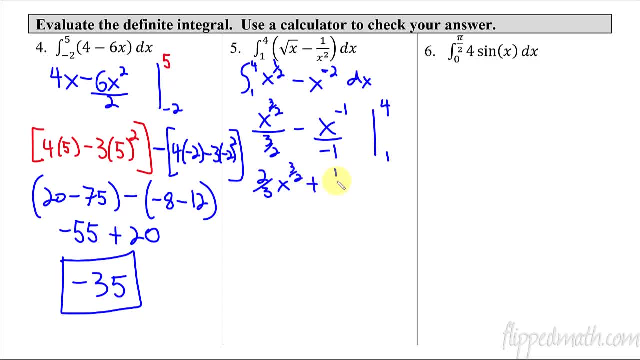 to simplify it even more. So this is 2x. I'm going to simplify this even more and I'm evaluating it from 1 to 4.. Okay, now let's go ahead and start plugging in these numbers. So the upper bound goes in first. 2 thirds, 4 raised to the 3 halves. Oh, I made a mistake right there. 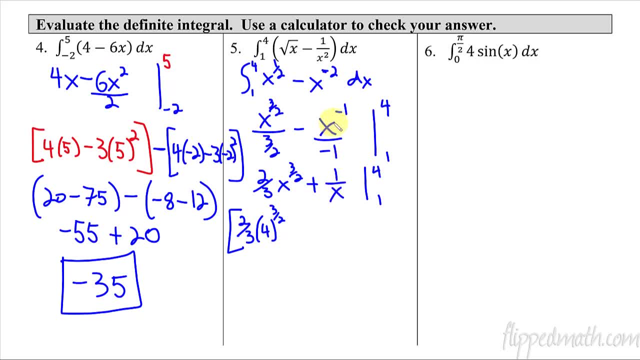 Somebody caught it. That wasn't a fourth, That was an x. I was ahead of myself And I had that supposed to drop down. Make that an x. Sorry about that. Okay. so now we say plus 1, fourth, 9 times 2x, which is x, 2x, 3x. 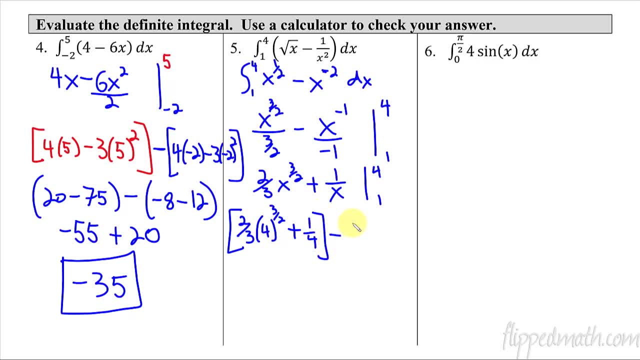 one-fourth bracket subtract. Now we'll plug in the one, So one gets plugged in here. That's easy. That's just two-thirds plus one gets plugged in there, one. Okay now, it's just simplifying these things. 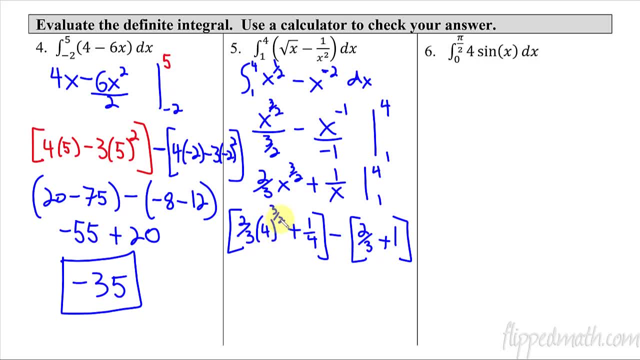 And I would give you a suggestion: Remember when you have this three-halves here, the two on bottom means square root. I would start off with that. So make that two-thirds times. the square root of four is two, and then two to the third. power is eight. 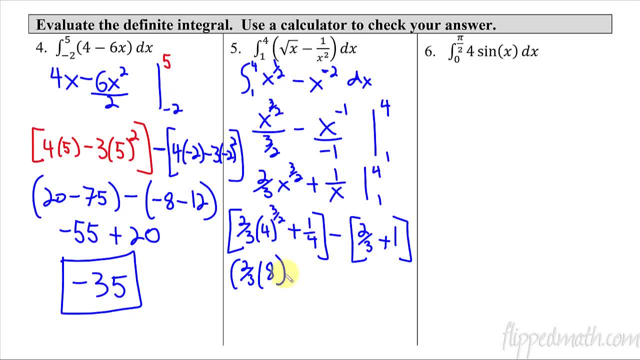 Makes it a lot easier if you do the bottom of the fraction first, for these exponents Plus one-fourth, And then this is three over three. plus two over three is five over three. Okay, now it's just a matter of going back to our elementary school. 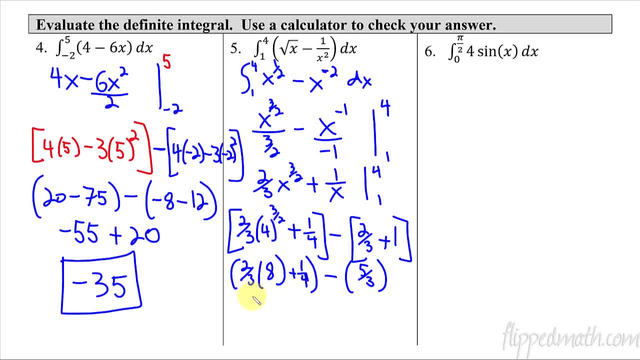 and remembering how to add fractions, So I'm just going to skip ahead on this one. Sixteen-thirds plus one-fourth minus five-thirds, I've got to get a common denominator of 12.. So that gives me 64-twelfths plus three-twelfths, minus 20-twelfths. 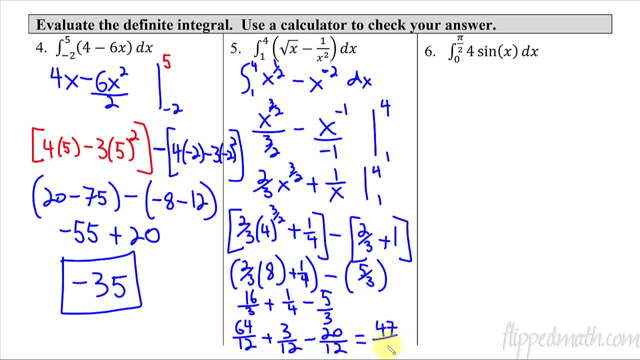 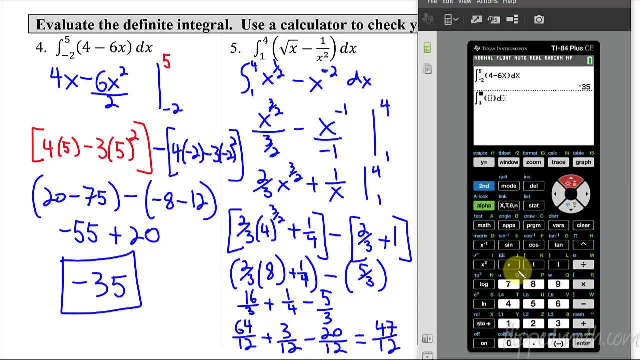 And then that all equals 47-twelfths. Now let's check our calculator, Math nine, Integral from one One to four, And then that is the square root of x minus one, divided by x, squared all with respect to x. 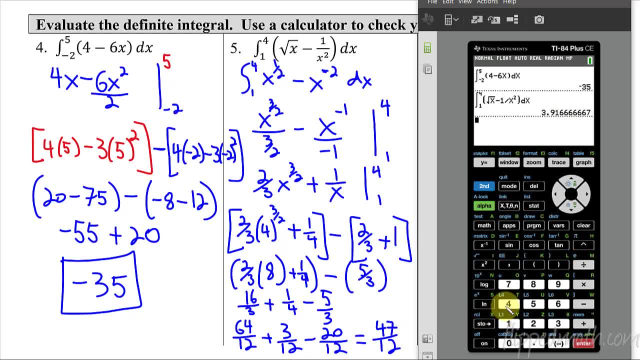 Okay, hit enter 3.91667.. Now, is that the same thing as that? Let's check 47 divided by 12. Enter. Yes, it is That's awesome. Okay, good, So we're good on that one. 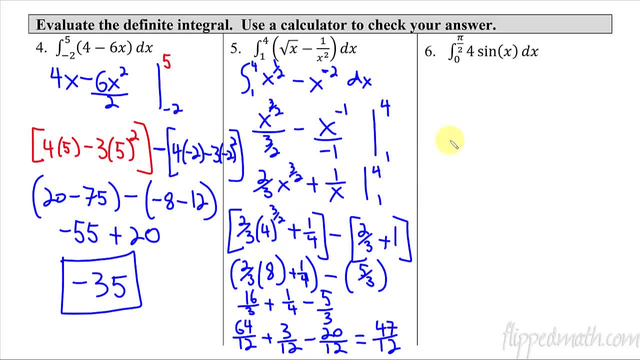 Thank goodness, that would have been awful. I did that one wrong. Okay, so now we go on number six. So we go. this four could actually just come out, if you want. Remember that property of that, properties of Integrals, so you can treat it like this: 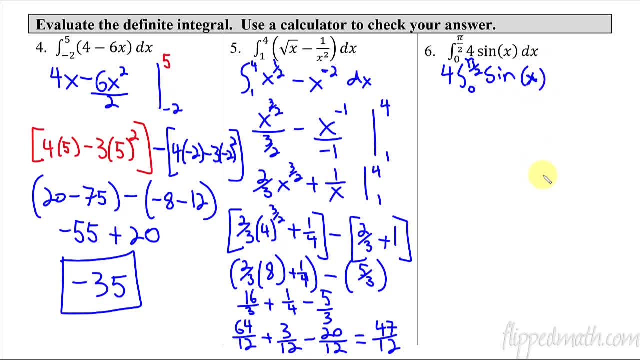 And now you're going to pause. That's right. Do this one on your own. So pause the video and then let's come back and see if you did it right. And you should have come up with just the number four. You can see what I did. 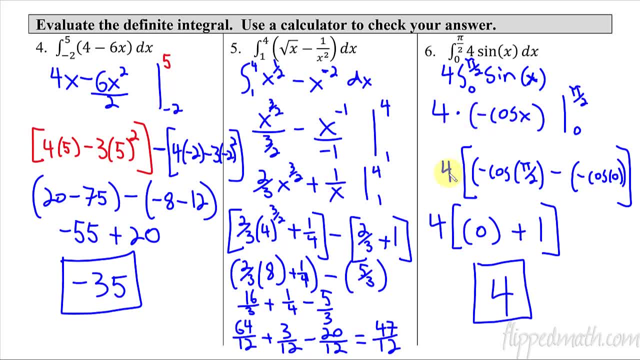 Follow my work here. You could also brought this negative. You could have brought it out with the negative four and just left it off on the side if you didn't want to do with the negative on the inside. So there's several ways you can manipulate this to work it out, but that's what you should have come up with was four. 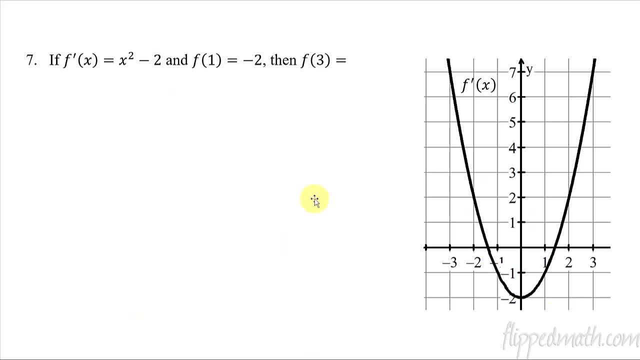 Okay, Last type of problem You're going to see in today's Practice, and that is when you are given the derivative. remember that the derivative represents the rate of change. So they'll give us the derivative And then we have one point of the original function. 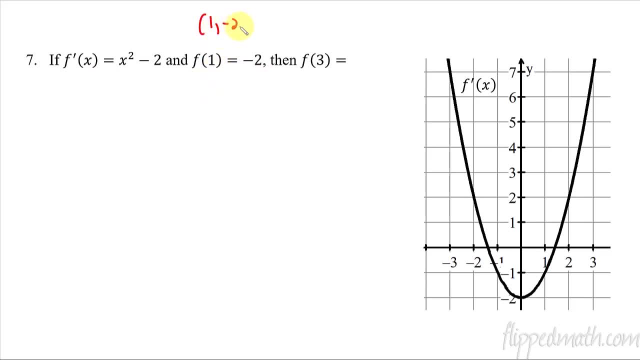 We know F of one equals negative two. So remember that's just a coordinate point: One common negative two. What they want to know is what is the Y value at X equals three. What we can do is what this? what we're trying to do is figure out the accumulation of change between one and three. 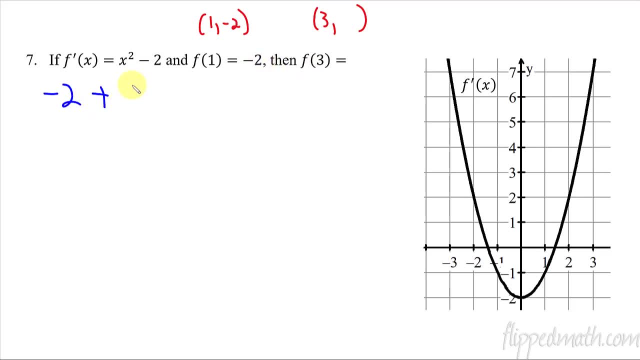 So we start at negative two and we're going to add the Integral of how much it's changed between one and three, And that only works if we have F prime. this has to be F prime right here with respect to X, And it is so F prime.